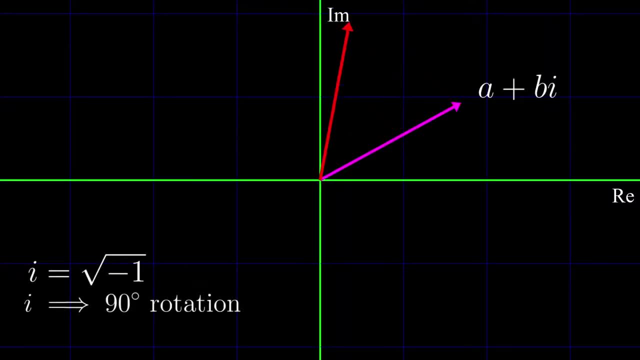 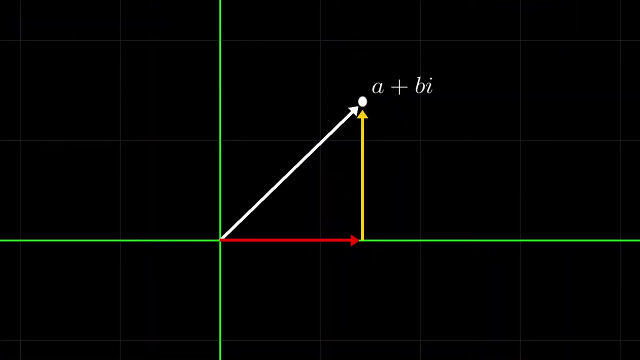 square root of negative 1.. You must have heard that multiplying a number by I has the effect of rotating it by 90 degrees in the complex plane. This is because when multiplying by I- the real part- the number is flipped counterclockwise to the imaginary line and similarly the imaginary 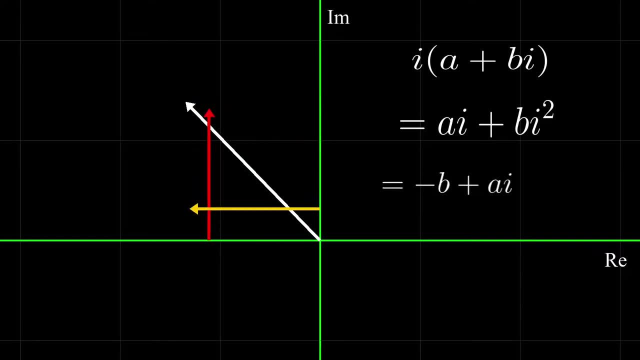 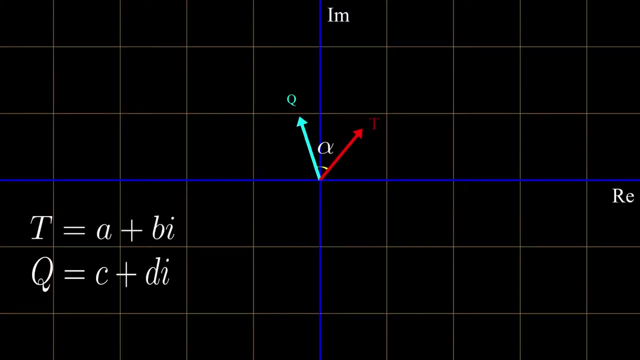 part is flipped counterclockwise to the real number line. as i times i or i squared is equal to negative 1.. Moving on here is some arbitrary point t equal to a plus bi on the complex plane. We need to rotate this point by some angle alpha, as shown here, to point q equal. 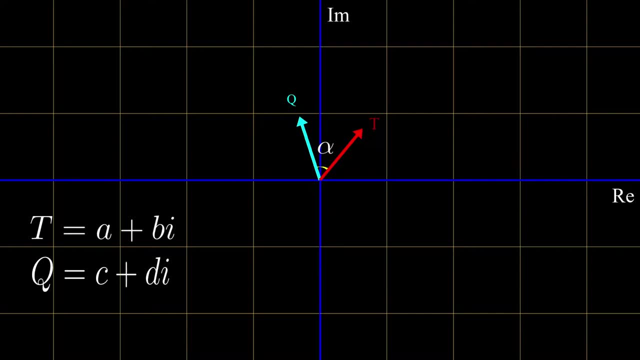 to c plus di. For now, this is just a rotation, so q and t are both of the same magnitude. What should we multiply t by to get to q? Well, remembering that vectors can be split into their subcomponents, here's one thing we can do: Duplicate t vector and scale one. 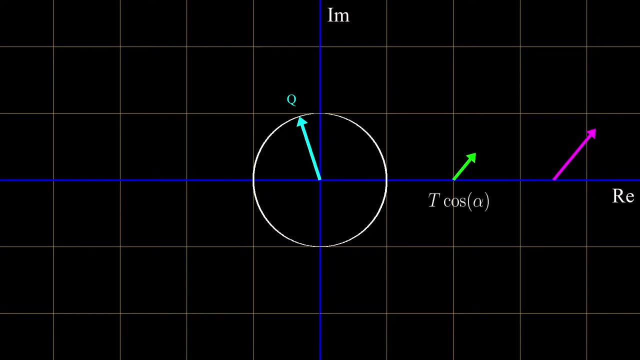 of the duplicates by cosine of alpha to the other duplicate. multiply it by i and then scale it by sine of alpha. Multiplying by i has the effect of rotating it by 90 degrees. Adding these two duplicates together, we can see that we have successfully. 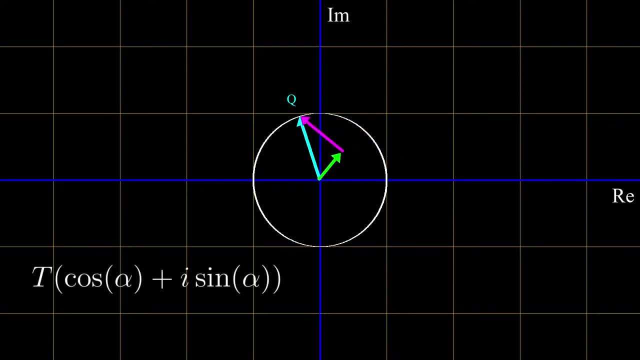 transformed point t to point q. What we just did is transform t to the subcomponents of q and thus adding these subcomponents gave us the point q. To make it more clear, let's change the perspective a little. We may rotate the graph such that 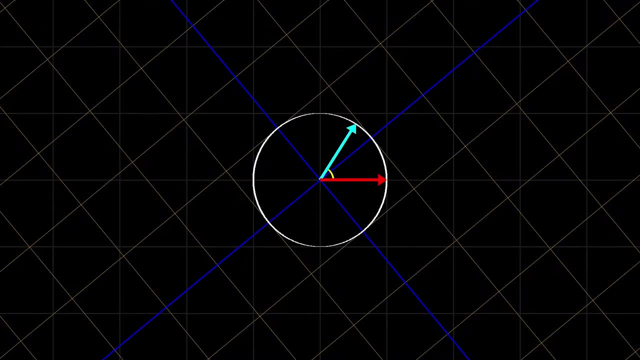 our original vector representing point t, appears to be the base of point q. We may now repeat the process mentioned previously. Note that the values of t and q will, of course, still be a plus bi and c plus di. this is just a change of perspective. When you rotate, 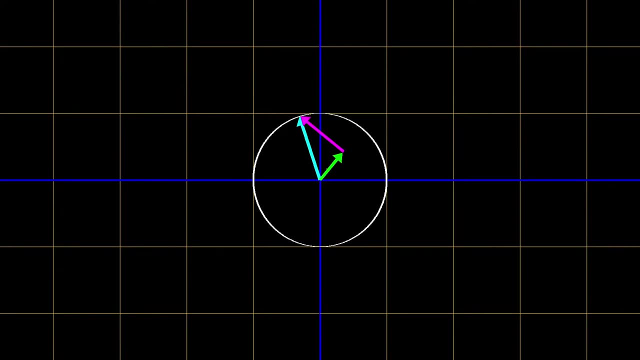 everything back to normal. we can see that we have successfully transformed t to q In terms of algebra. we can see that we multiplied point t by cosine of alpha plus i times sine of alpha. This implies that any point x can be rotated by some alpha degrees. 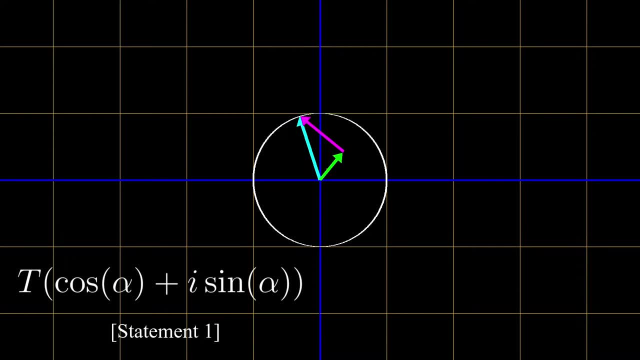 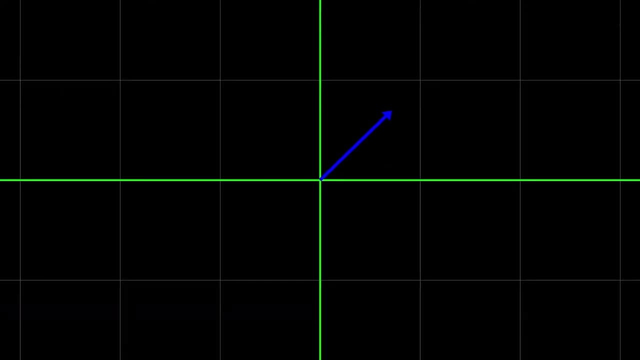 simply by multiplying by cosine of alpha plus i times sine of alpha in the complex plane. One last thing: we know that cosine of theta plus i times sine of theta, where theta is the angle made with the real number line, just represents the unit vector, that is the set of all points with magnitude 1.. This 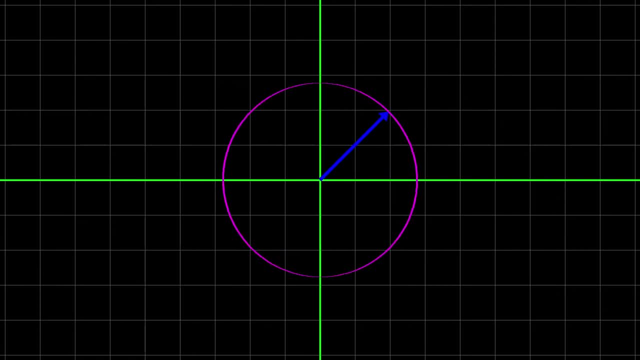 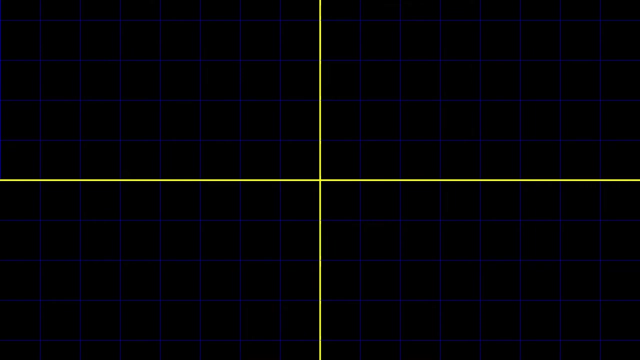 is extremely important as all points in the complex plane are just a scaled form of this unit vector, That is, any point a can be represented as cosine of theta plus i times sine of theta, times the magnitude of a, where theta is the angle point a makes with the real number line. So finally, when you're multiplying, 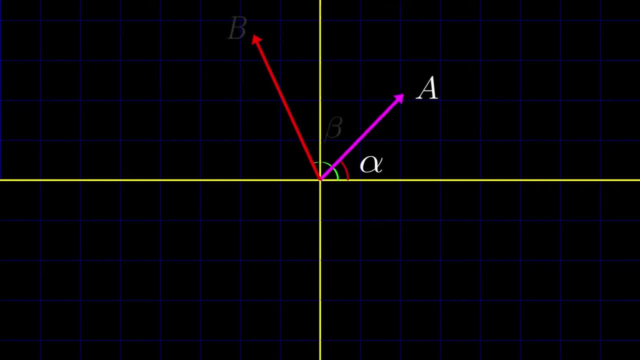 two complex numbers, a and b, of different magnitudes and of angles, alpha and beta respectively. they can be broken down like this: Magnitude of a times cosine of alpha plus i times sine of alpha, times magnitude of b times cosine of beta plus i times sine of beta. What that means is that a unit vector of 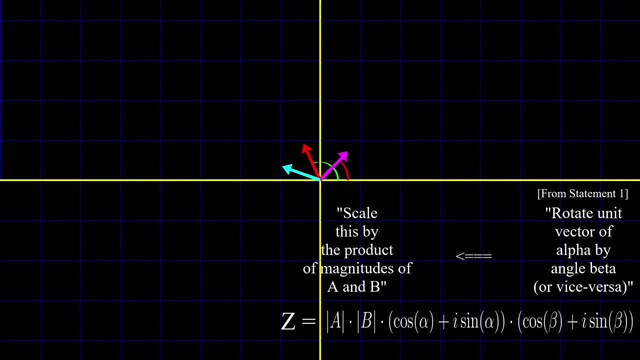 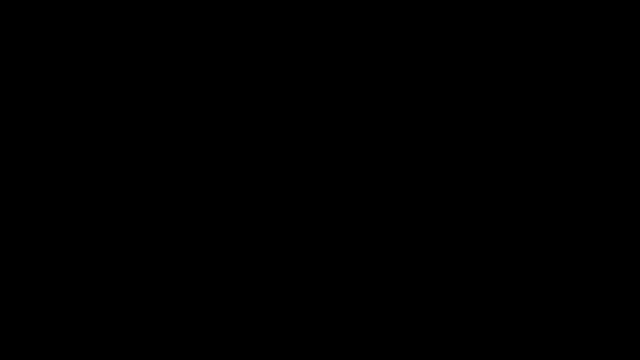 angle alpha is rotated by angle beta or vice versa, and then scaled to the products of the real number line And therefore, when two complex numbers are multiplied, the new value formed is set to be a scaled and rotated version of them. Complex numbers are extremely useful. They 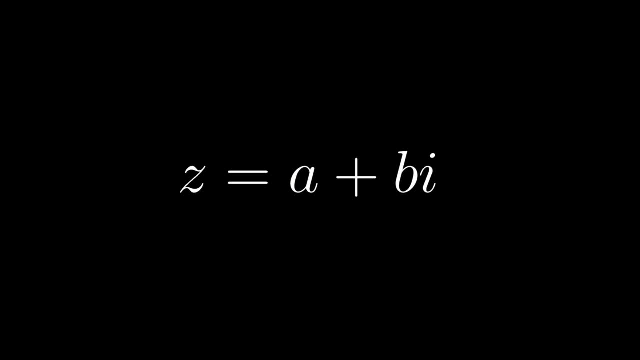 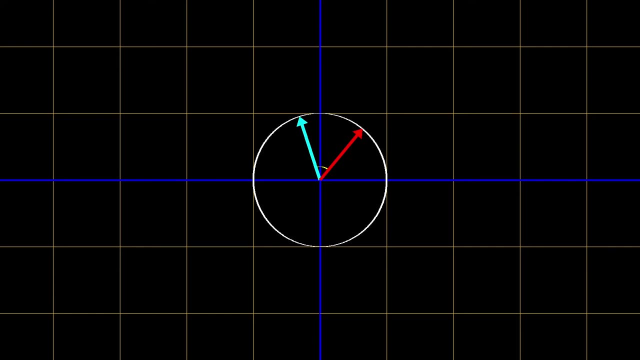 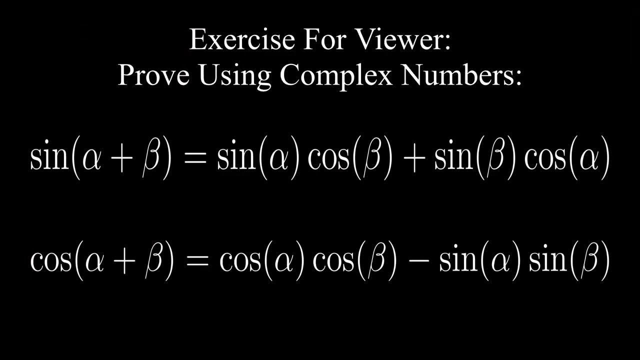 are used in many fields, ranging from quantum physics to computer science. They are also very helpful in computer graphics. In fact, in this video, the animation of vectors and graphs were made with the help of complex numbers. Before you go, here's a fun little exercise that you should try by yourself, Using what 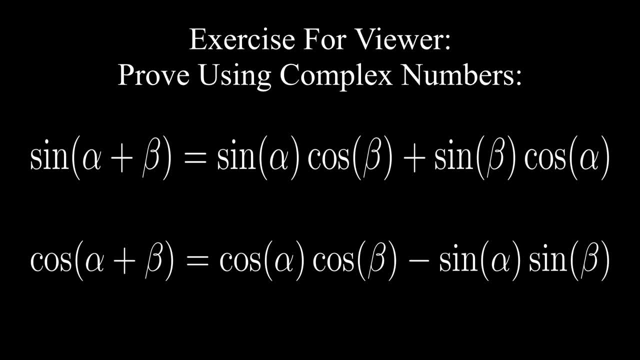 you learned in this video, try to prove the angle sum property of sine and cosine using complex numbers. Thank you very much for watching. I hope you found this video helpful.